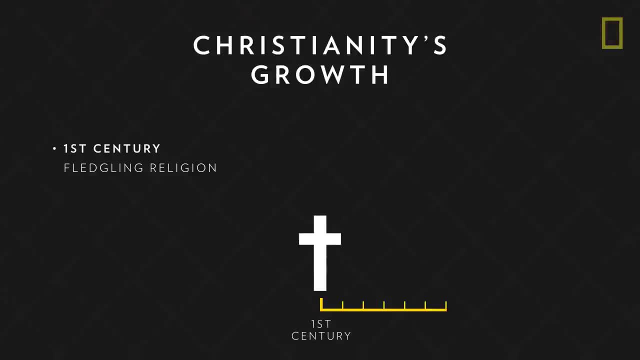 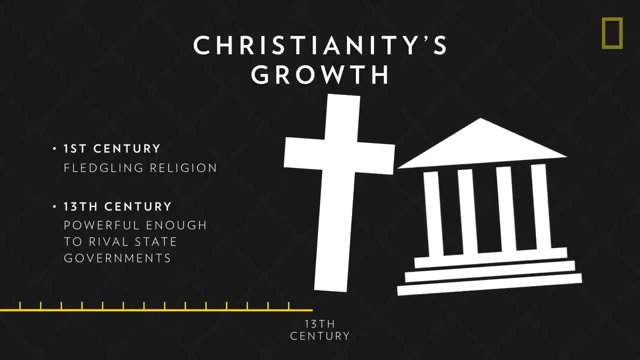 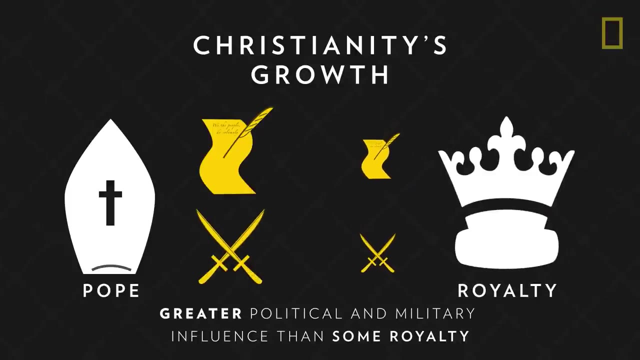 Christianity, which began as a fledgling religion in the first century, had grown by the 13th century into an institution powerful enough to rival state governments. For instance, the pope, then the leader of the Christian church, had greater political and military influence than 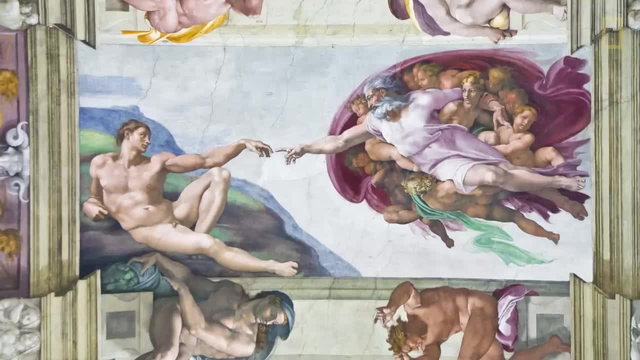 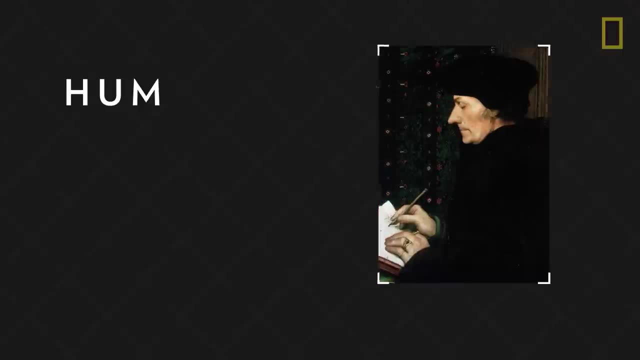 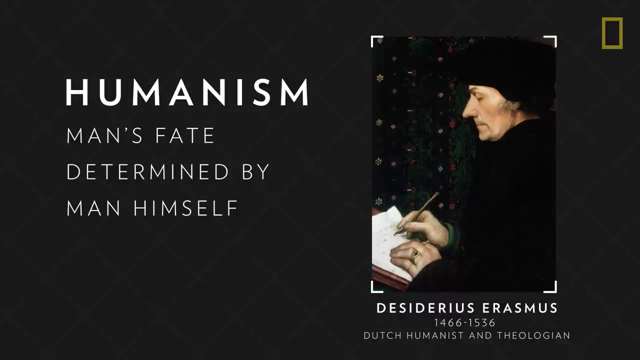 some emperors and kings. This tension was exacerbated by the transformative social and intellectual period known as the Renaissance. In particular, this period involved the rise of humanism, a philosophy that shifted man's fate from being determined by religion and religion itself. The Renaissance was a period in which humanism and religion 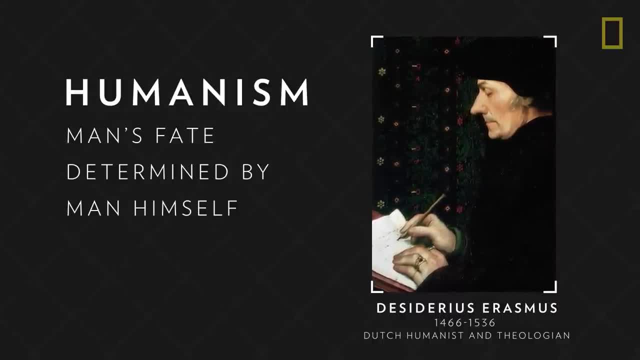 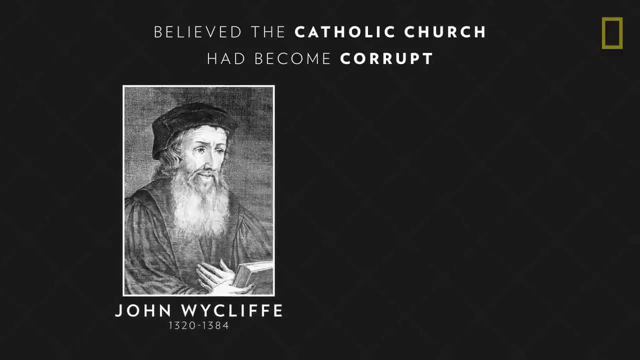 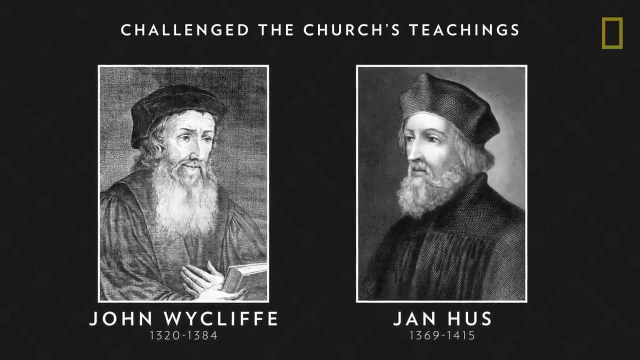 were divided by religious doctrine to being determined by man himself. Additionally, some within the church believed it had become increasingly corrupt. Priests like John Wycliffe of England and Jan Hus of Bohemia challenged the church's teachings, which they believed had strayed away from the Bible. However, one of the most well-known advocates for a 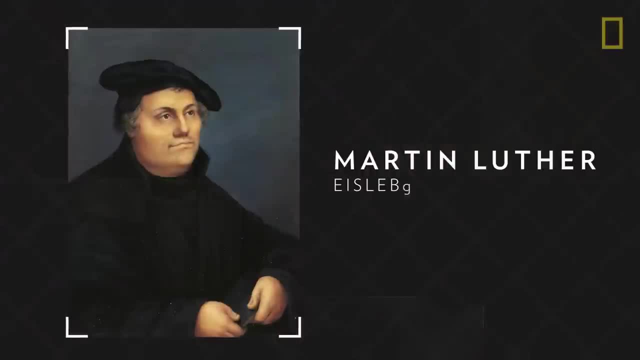 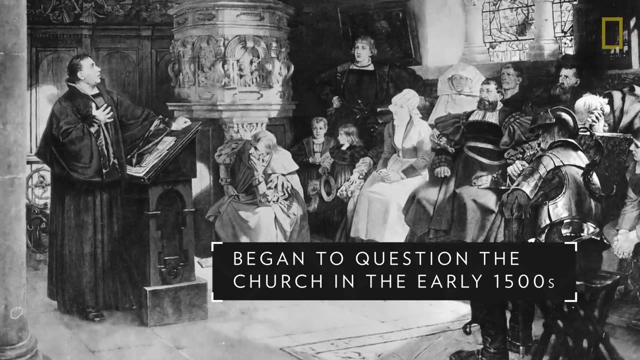 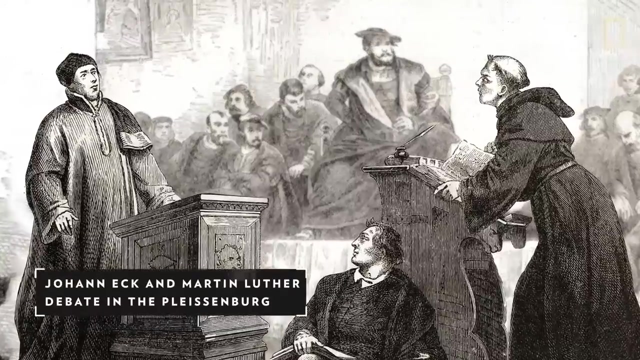 Reformed Christian church was a German priest named Martin Luther. Martin Luther began to question the church in the early 1500s. He believed it was abusing its power and disagreed with some of its practices. For instance, he challenged the church's doctrine that stated the pope, not the Bible. 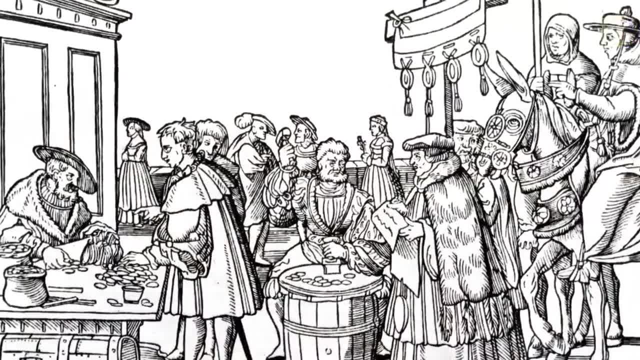 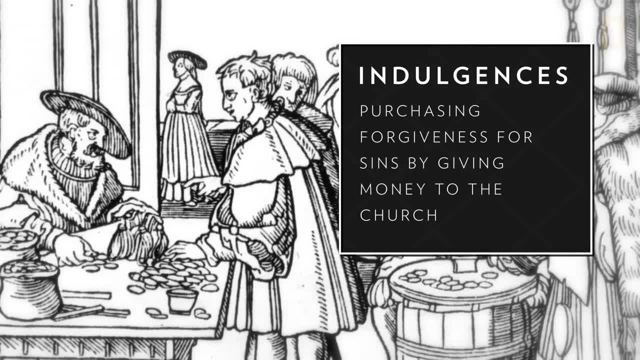 was the ultimate spiritual authority. Plus, he criticized the church for selling indulgences, the practice of purchasing forgiveness for one's sins by giving money to the church. Luther believed the church needed to revise its doctrine by returning to the Bible's teaching. 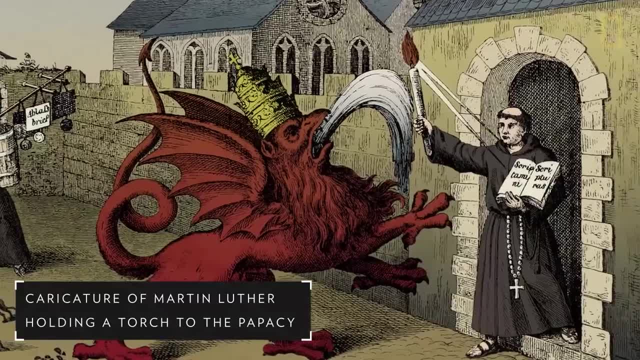 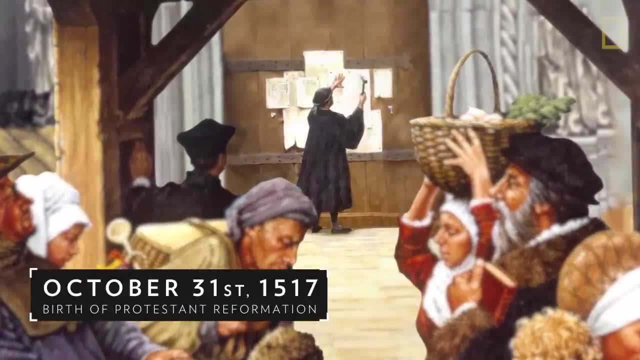 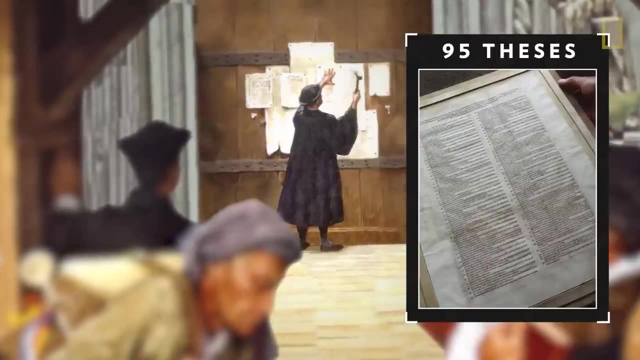 and by saying that salvation could be granted by faith in Christ alone. So on October 31st 1517,, Luther took a stand In what's considered the birth of the Protestant Reformation. Luther is said to have nailed 95 theses or arguments against the church. 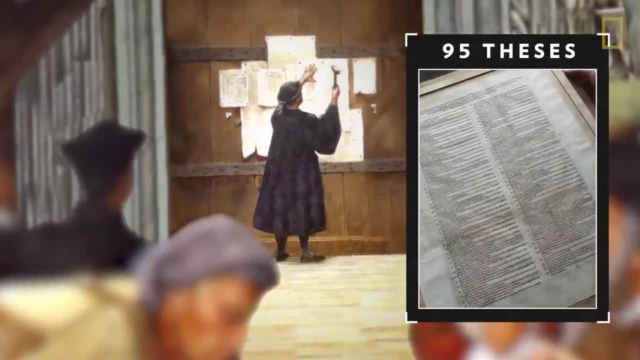 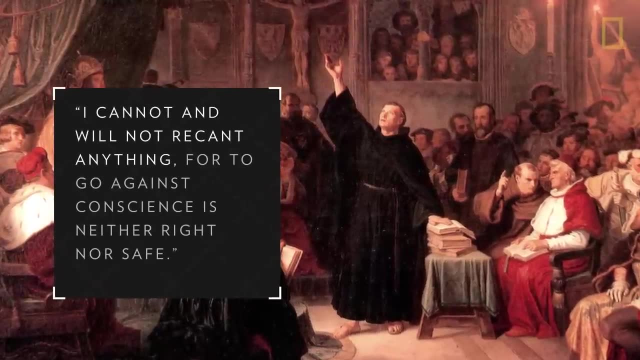 onto the door of Castle Church in Wittenberg, Germany. Luther was later put on trial in front of church officials to defend his theses, but it is not known how many of theses Luther wrote. But in January 1521, the church declared Luther a heretic and excommunicated him.